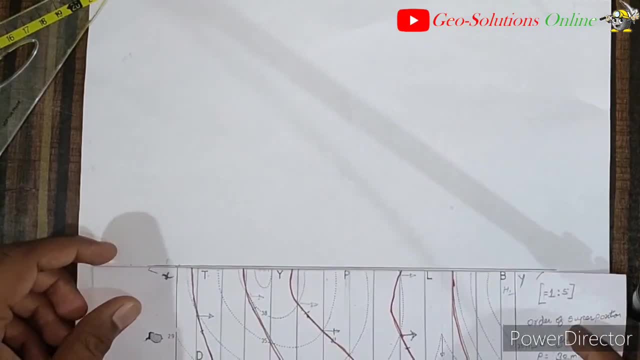 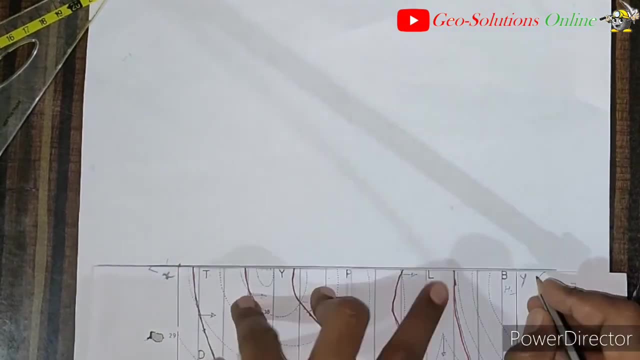 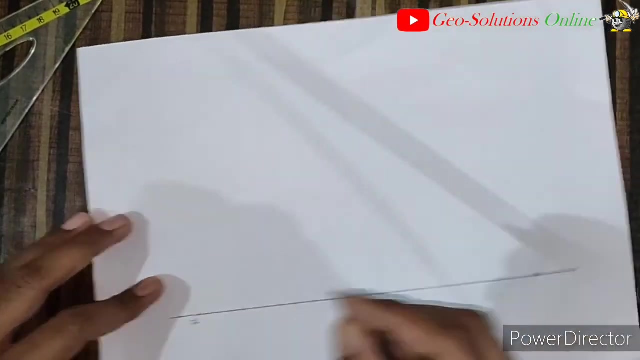 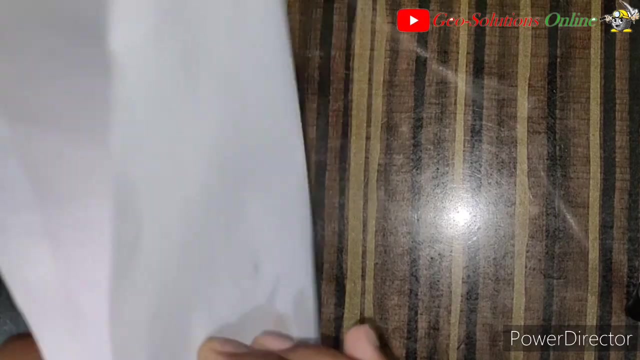 With the help of scale. Then we will place the folded map and we will mark the point X and point Y on the line drawn on the plain paper And this line will be called as line of axis or plane of axis. Okay, Then again we will join the point X and point Y on this plain paper. 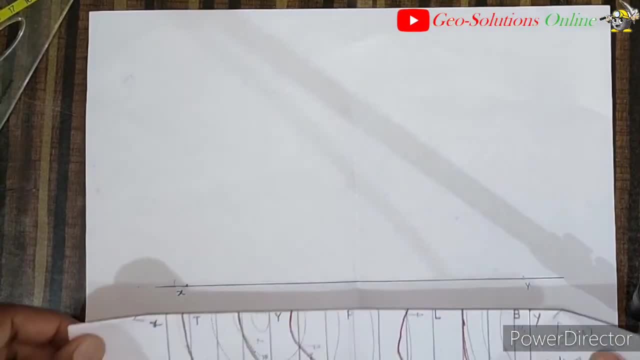 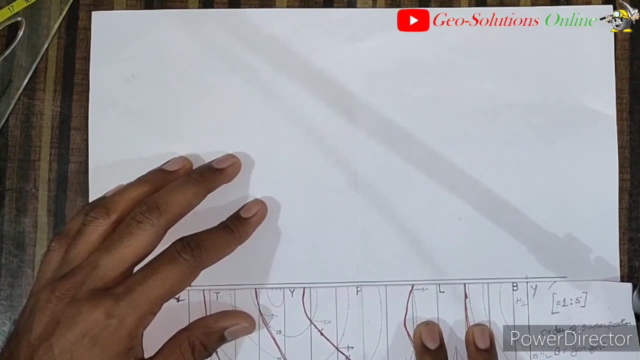 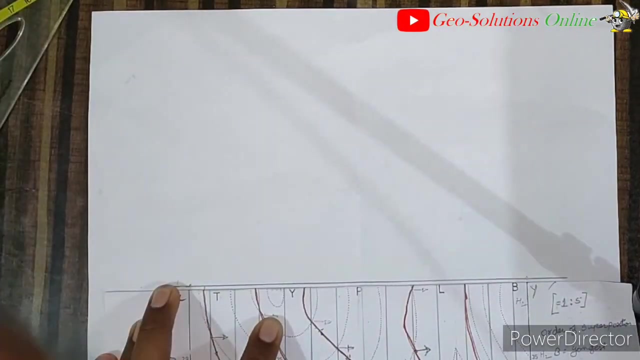 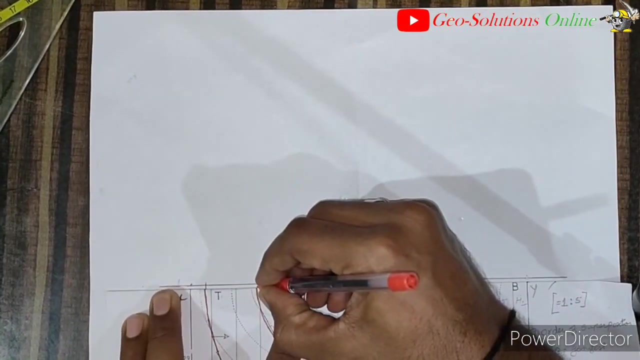 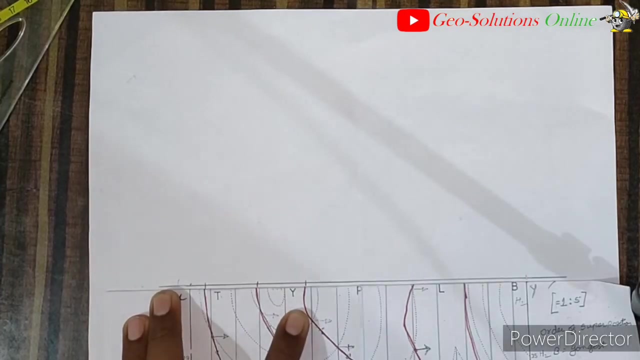 to get the center point of the axis. then we will keep the folded map along the axis to mark the features on the map. then we will mark the all the bedding planes on the map. okay, so you may use different color paint to plot or to mark the bedding plane too much. so in this way we had marked all the bedding planes. 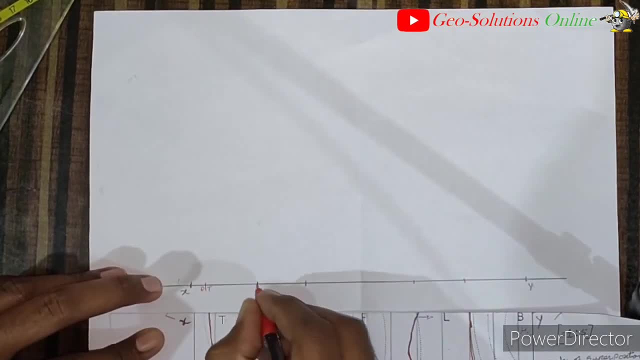 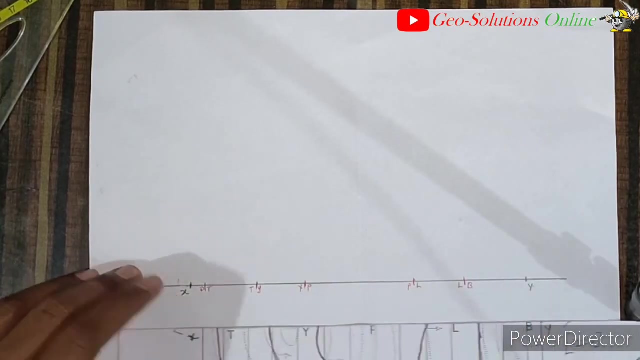 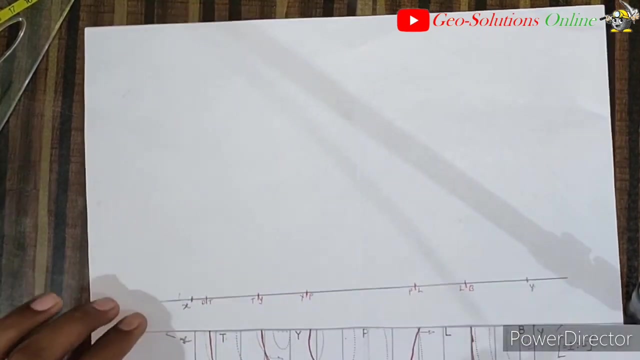 on the axis line. so bidding plane points are marked. then we are labeling the bedding plane points. the bedding plane DT, DY, YP, bl and lb are all are marked and point X and point Y are also marked. so further we have to draw a line vertical on the these axis line. okay, 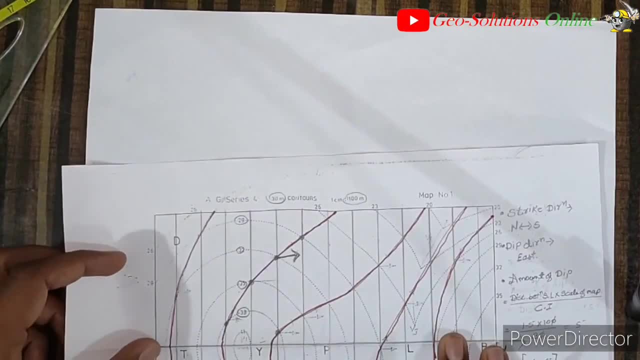 at point X and point Y as a reference line. so, nearer to the X, the contour is of Y plus 1 of the vertical is of Z1 and the length of this line is of factor x. okay, and then we will draw this vertical line on the hacia siz line. okay, so 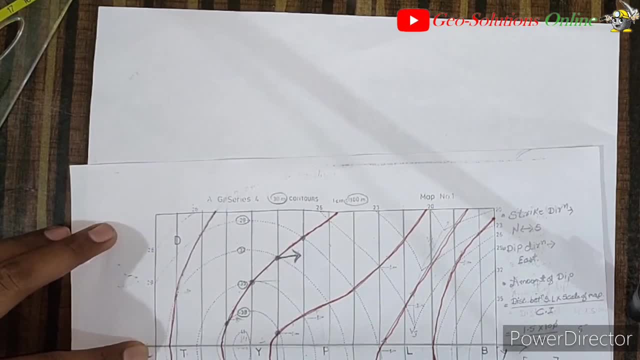 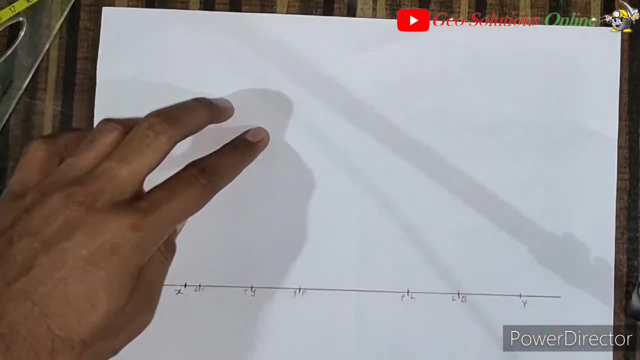 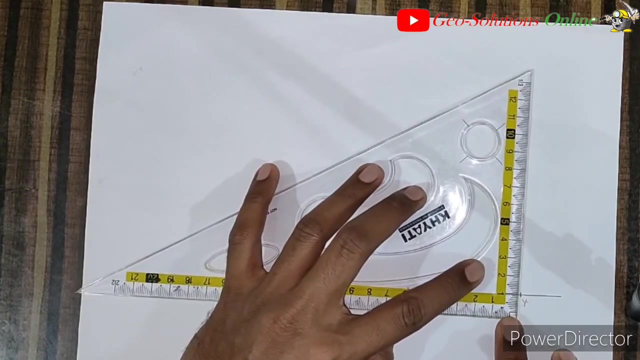 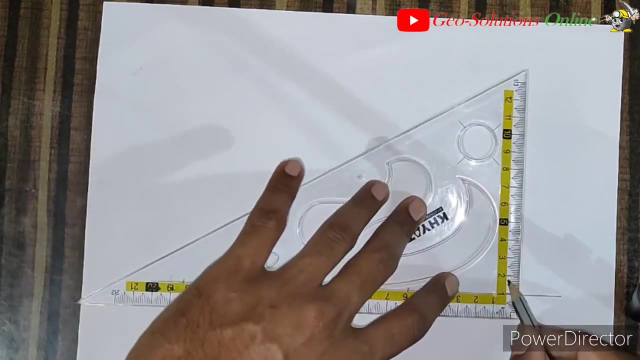 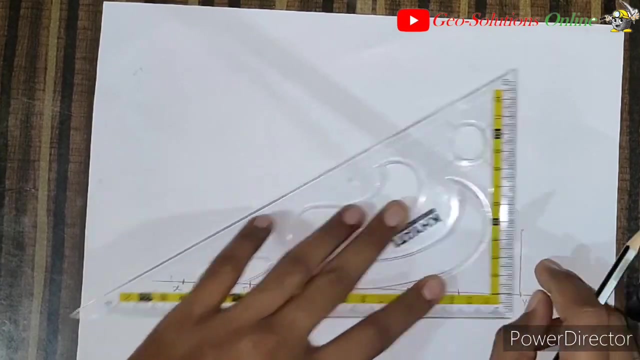 to 90 meter and nearer to the Y, the contour line is of 350 meter, so we will consider this as a reference point for the line. okay, so at the both side, with the help of scale, we will draw the perpendicular line on the axis. okay, so on y-axis, the line length must be 3.5. okay, because the 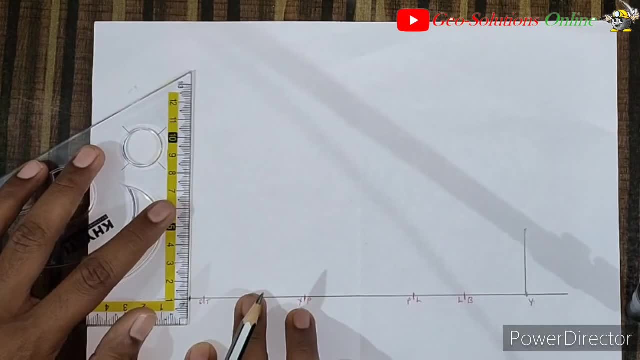 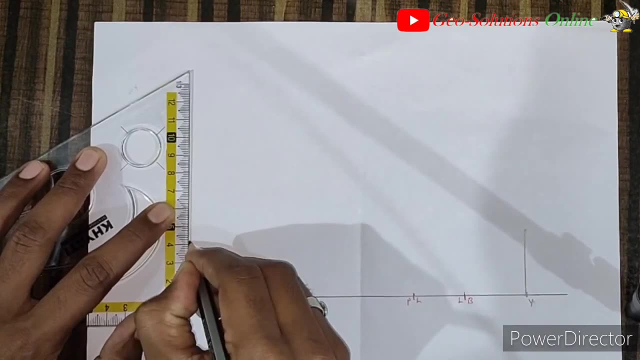 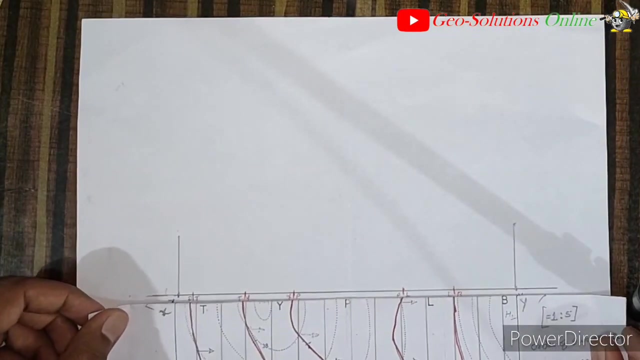 nearest contour is of 350 meter and our scale is of 1 centimeter equals to 100 meter, so that's why 3.5 centimeter and towards the x-axis, the nearest contour is of 320. so now we are going to plot, or marked, all the. 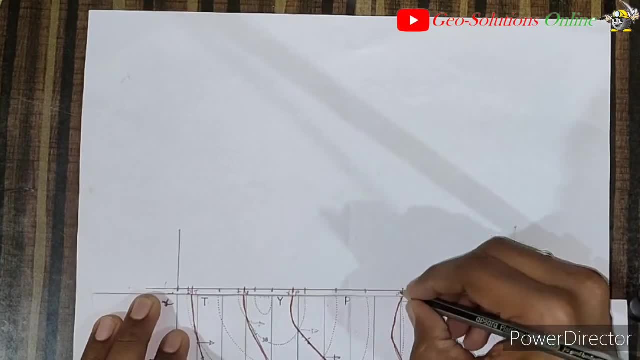 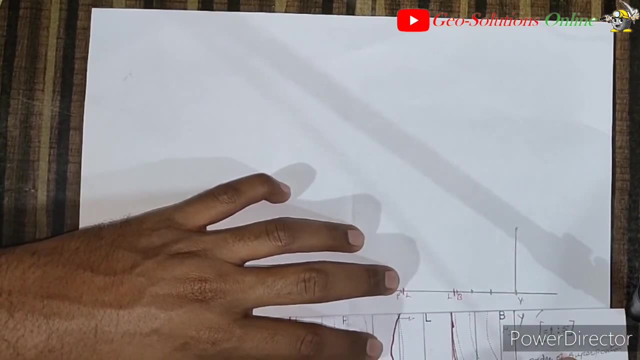 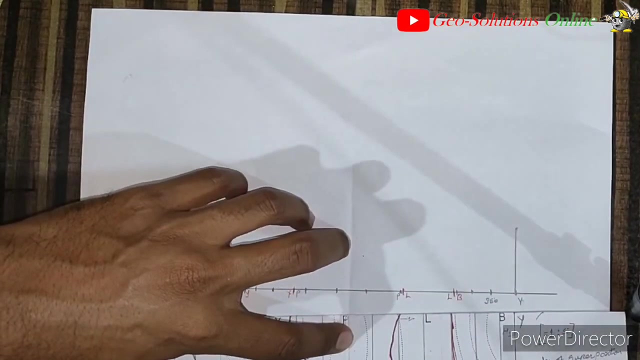 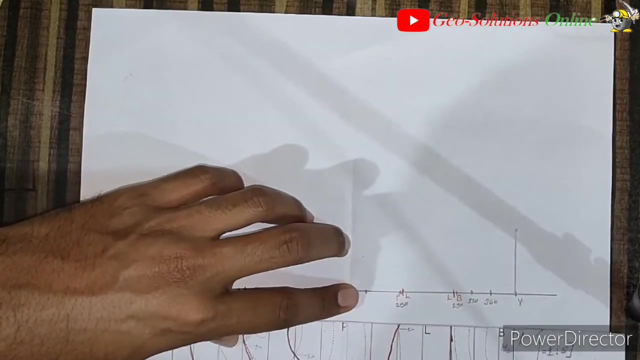 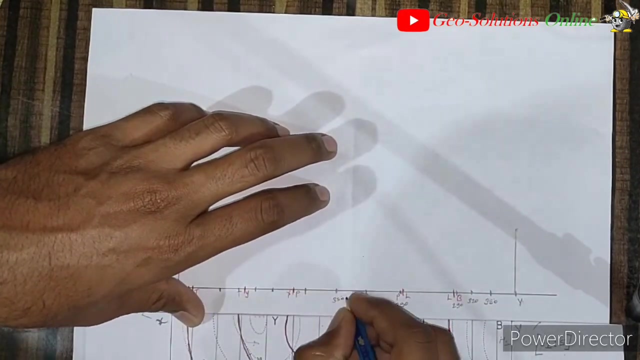 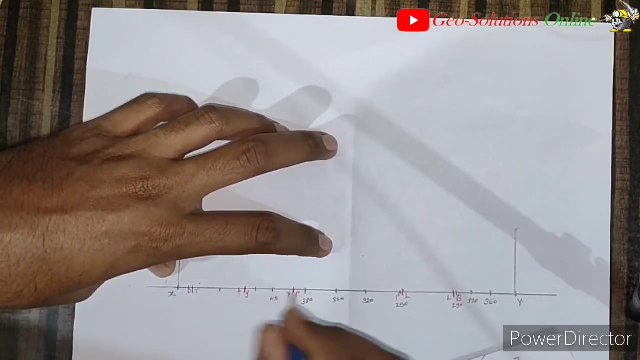 contour lines as well as their values. okay, all control line points are marked, so we will label it with its value. so first control line is of 350 meter to 90 meter control point, then again to 90 meter, control point 320, then next one is of 350- 380, then next one is for 10, another for 10, next one is of 380. 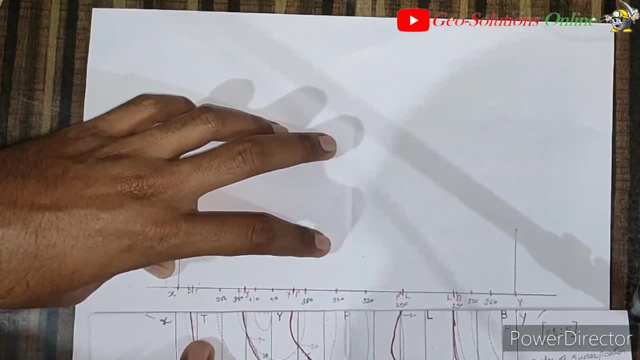 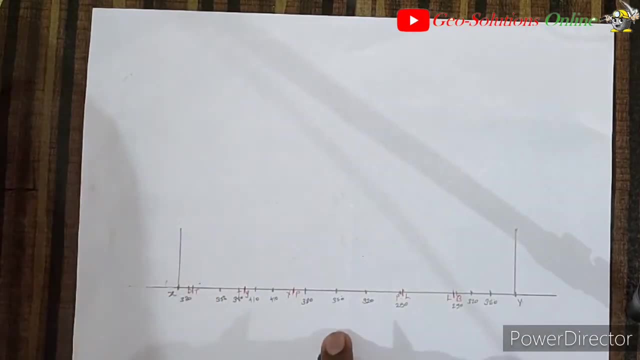 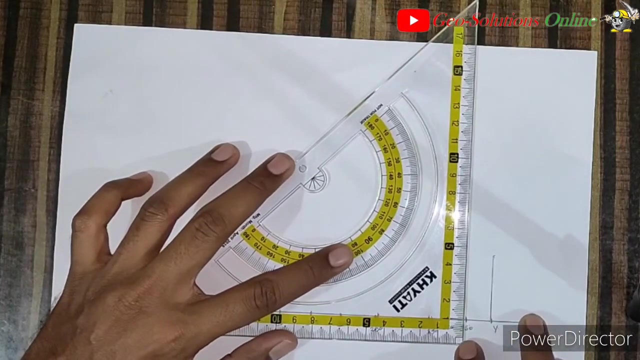 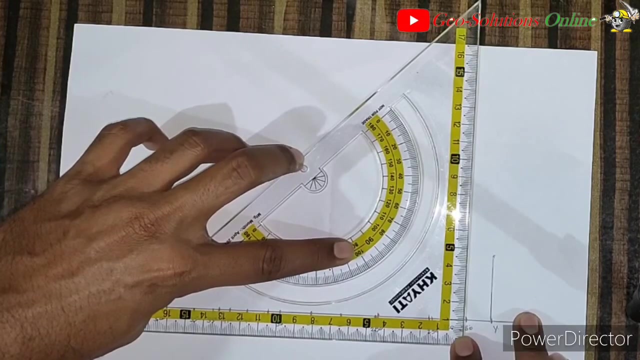 you're correct, then 350, then last one is of 320. in this way, we had labeled, marked and labeled all the bedding planes, all the control points, as well as their values. then now you are going to determine which code you're going to use, because if you 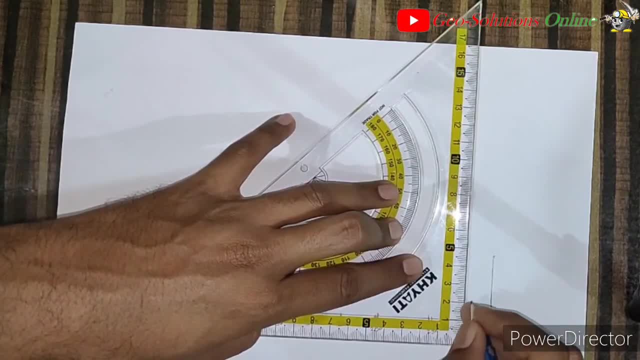 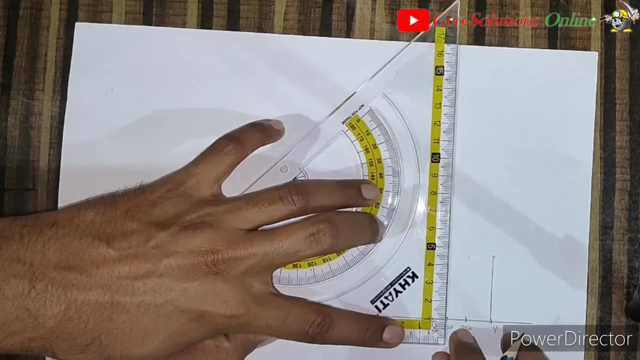 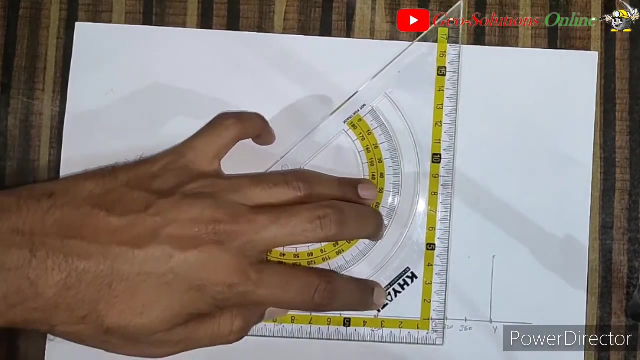 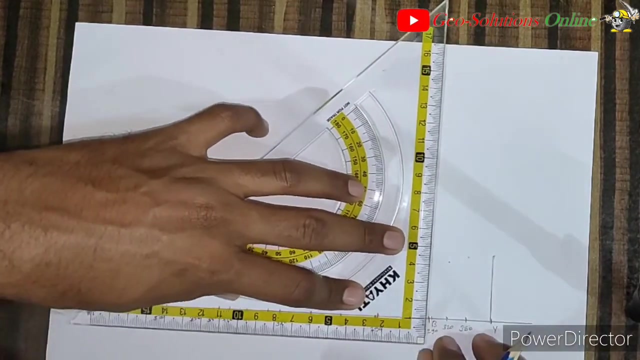 think of a set square. so you guys know how to do it, the shape of the set. with the help of this set square we are going to mark the point exact perpendicular above the axis point. whatever the value is of we are going to is of 320 meter, then we will plot it on 3.2 centimeter. the next point is of 290. 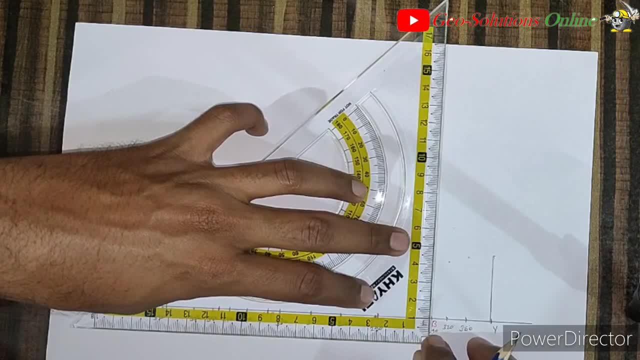 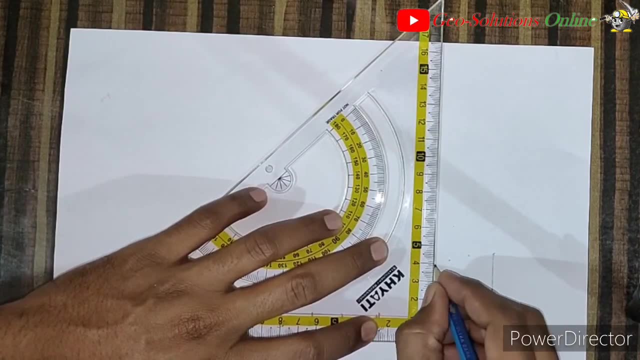 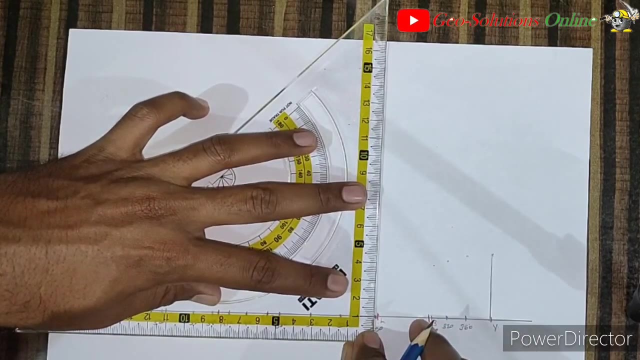 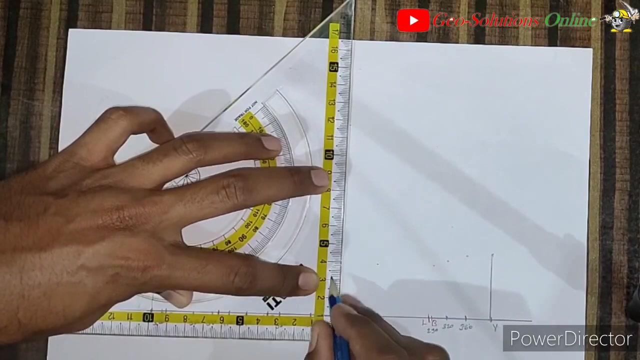 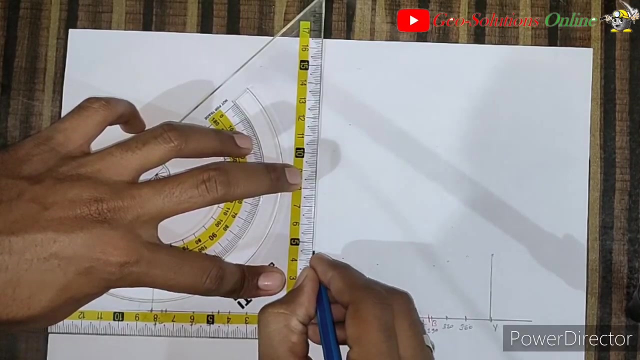 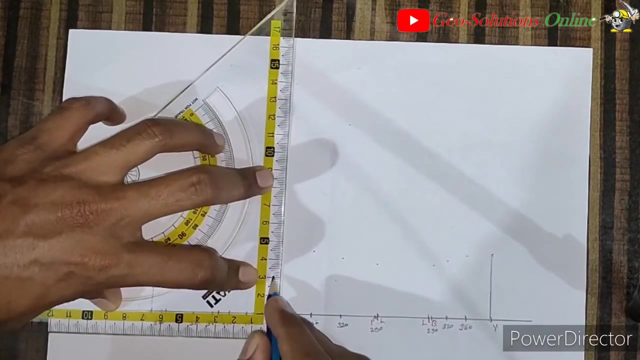 meter, that is 2.9 centimeter. it's okay, so carefully mark the point sectabo perpendicular to the axis line, then next point is of 2.9 centimeter, 3.2 centimeter, then next one is of 3.5 centimeter. cause our scale is of 1 centimeter equals to: 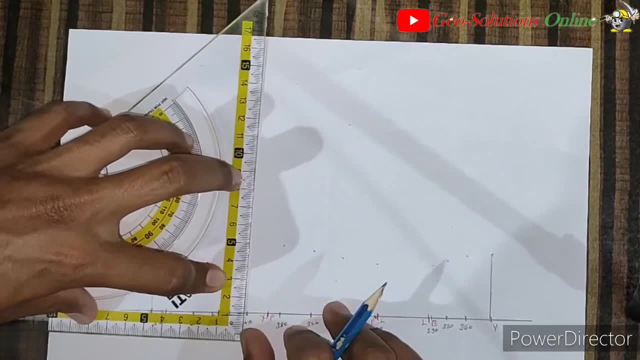 100 meter. okay, so we will plot it on 3.2 centimeter, then we will plot it on 3.2 centimeter. so 3.3, 50 meter equals to 3.5 centimeter. so next one is of 380, that is. 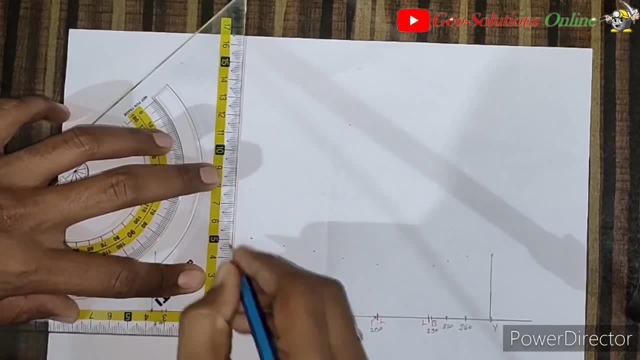 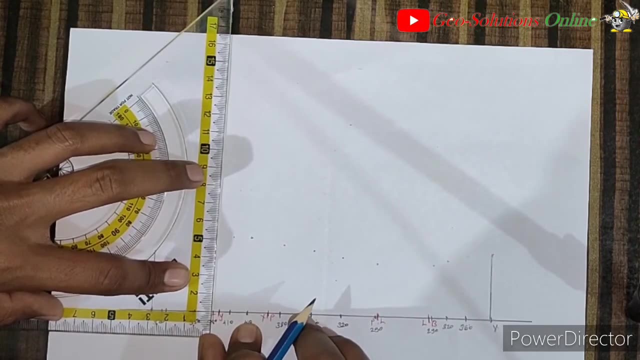 3.8 centimeter, the next one is of 14, that is, 4.1 centimeter. next one is also 4.1 centimeter, the next one is of 3.8 centimeter, then next one is of 3.5. 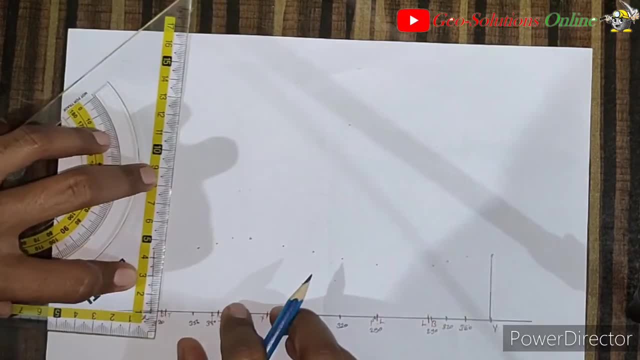 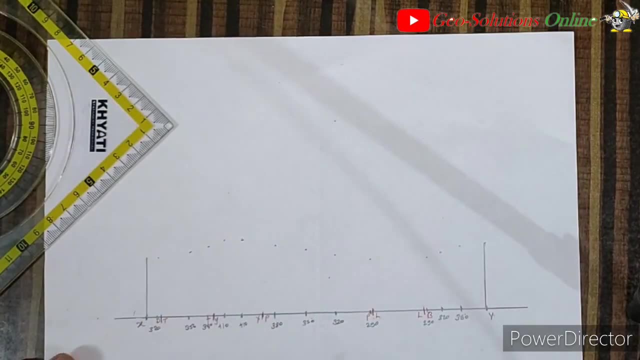 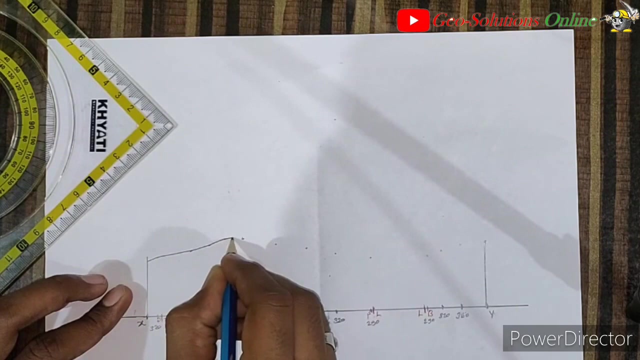 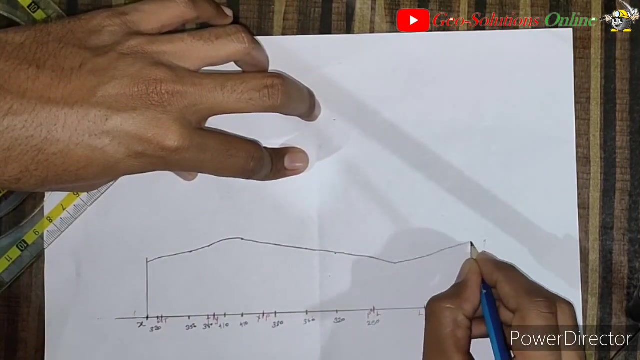 centimeter. the next is 3.2 centimeter. okay, this was the last one. so in this way we have plotted all the contour values and point above the axis line of axis pencil. with the help of pencil we will join each and every point by free hand. in this way we have plotted. 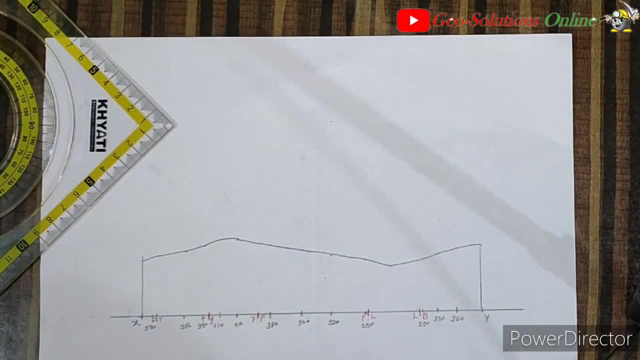 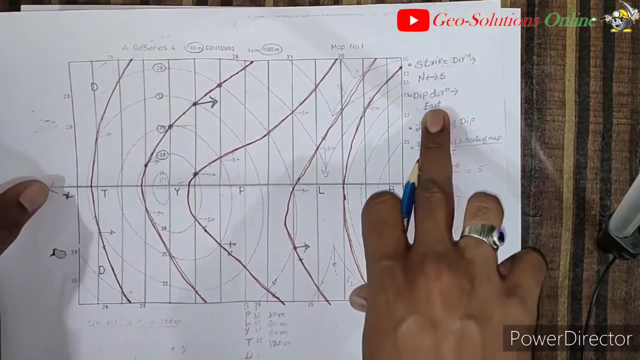 our section of map number 1. this map number 1 contains two isolated hill. one is complete isolated hill and other is one is a half portion of isolated hill. deep direction: we had already determined the deep direction means the amount, the angle of inclination with respect to the horizontal plane, so the amount of 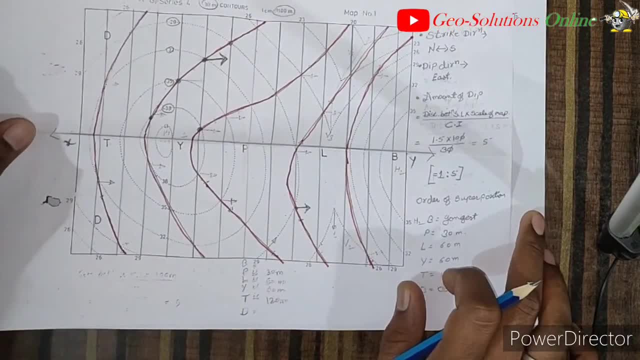 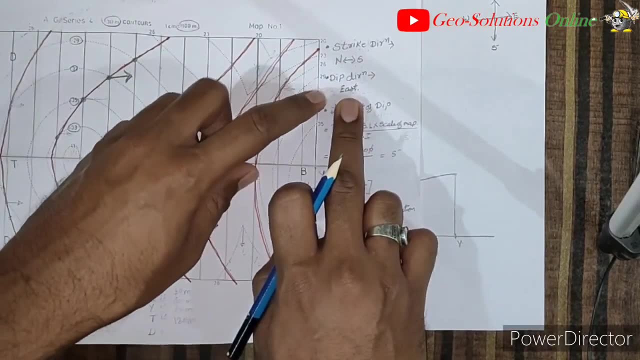 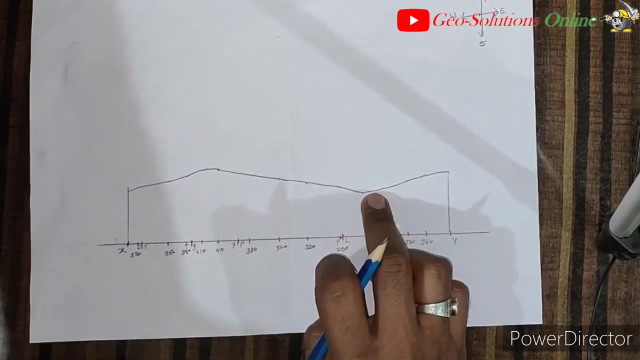 inclination of the beds with respect to the horizontal plane is the deep direction, and we had already determined the deep direction previous lecture. that is, deep direction is towards east side and the amount of deep is 5. so in ratio we will, we had already calculated. the amount of deep is equal to 1, is 1 is to 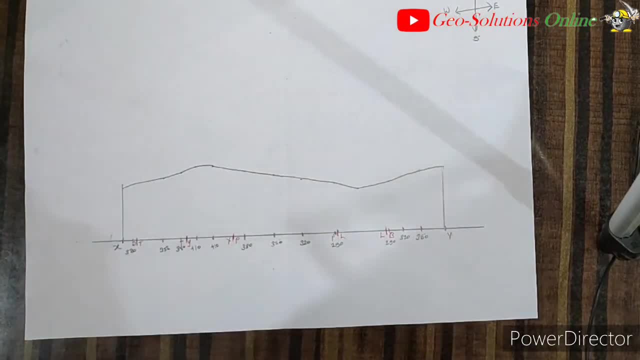 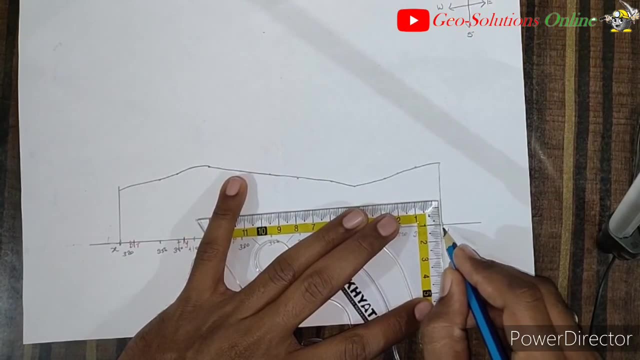 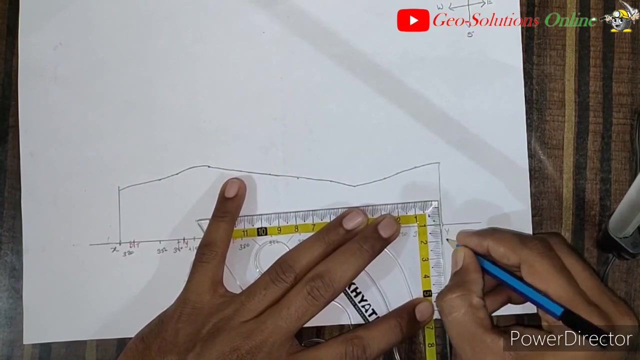 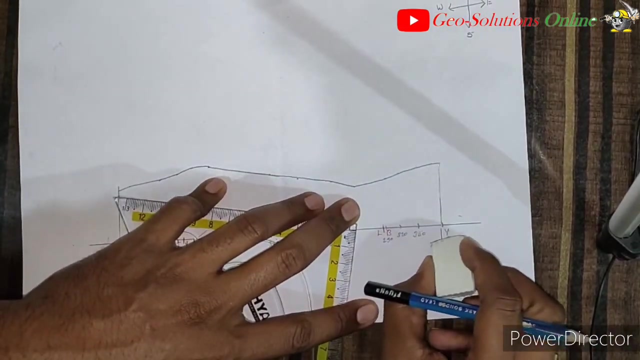 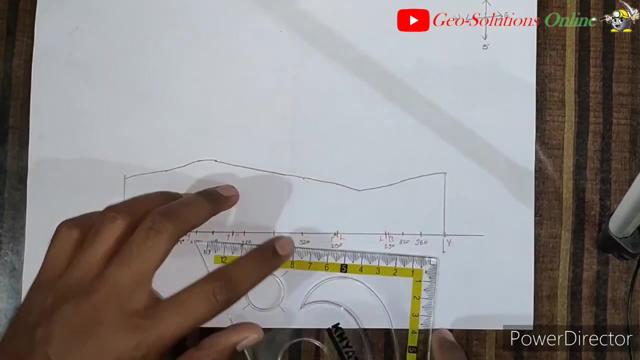 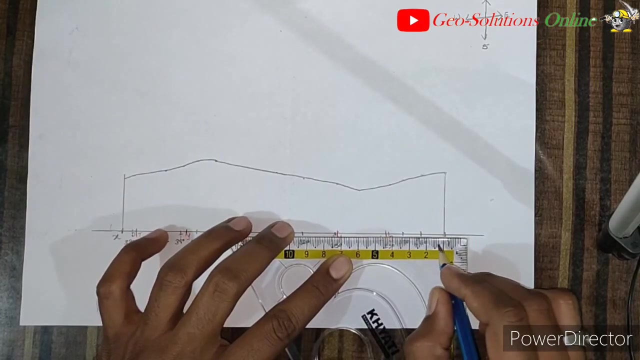 5, then in the east direction. so sorry, y point is in the east direction. so so, first of all we will draw a line of 1 centimeter, exact, okay. so 1 centimeter line is plotted for the inclined angle. then we will plot 5 centimeter from East: 1, 2, 3, 4, 5, okay so. 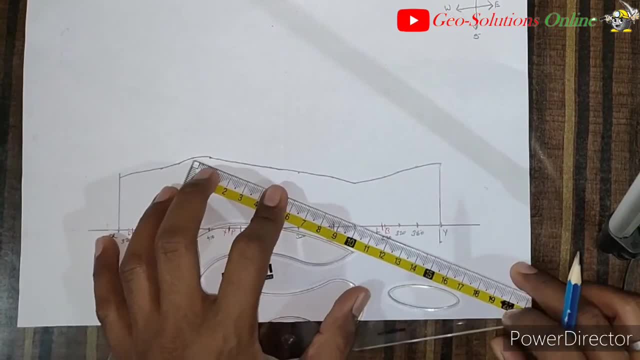 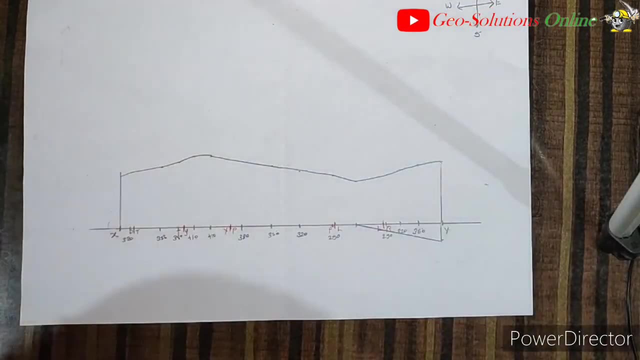 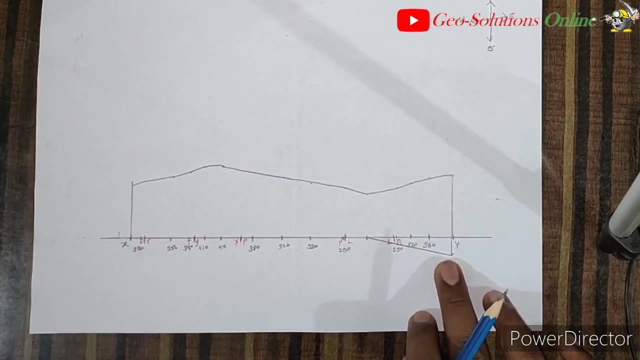 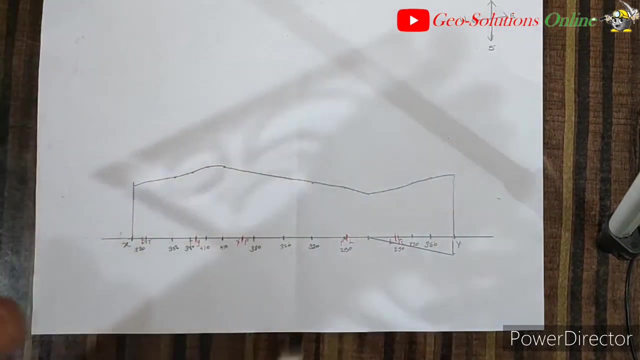 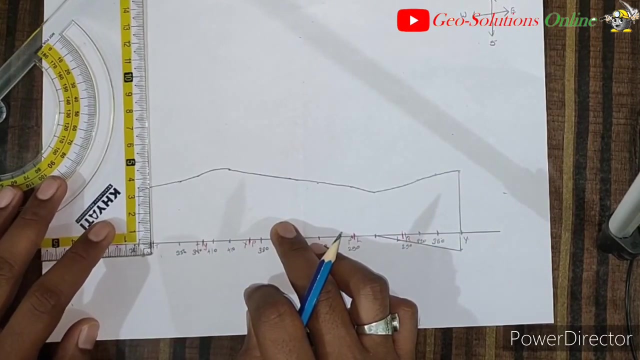 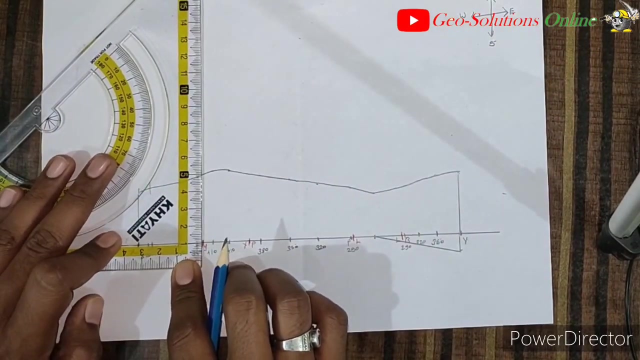 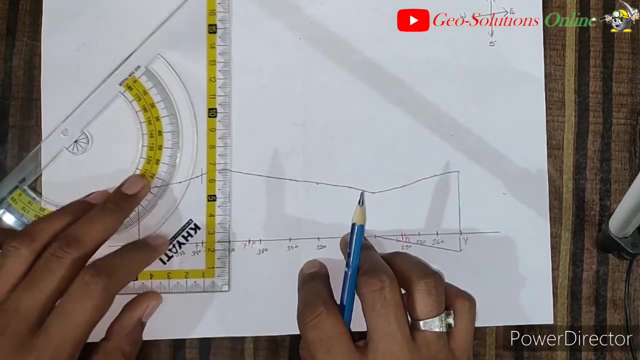 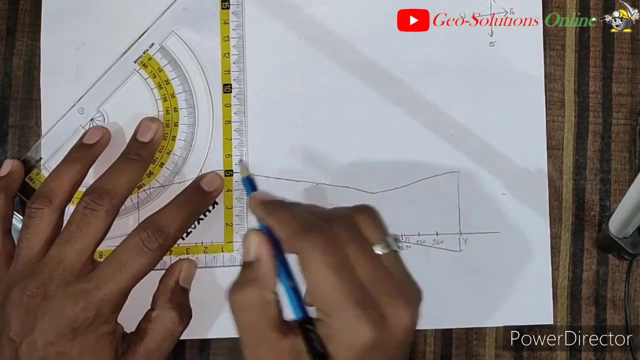 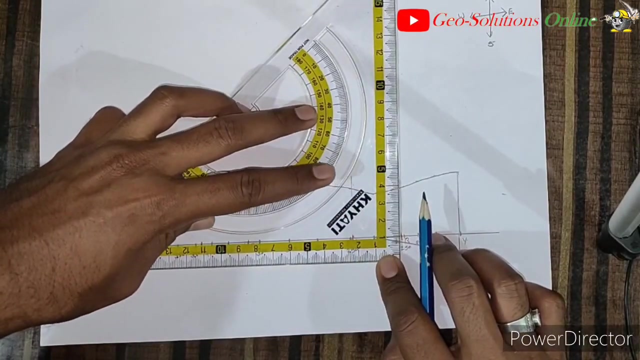 this is our, so join these two points. so in this way we had marked our reference of deep angle. okay, so we have to mark our bedding points on the section. we have to mark our bedding points on the section. try to mark exact. you may use the ruler scale. 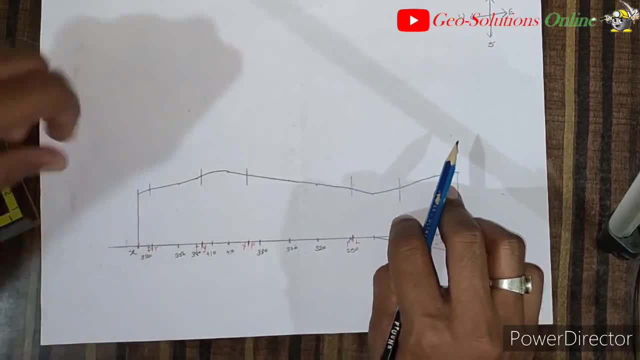 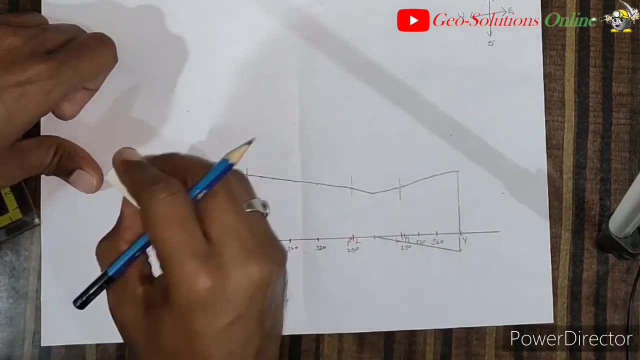 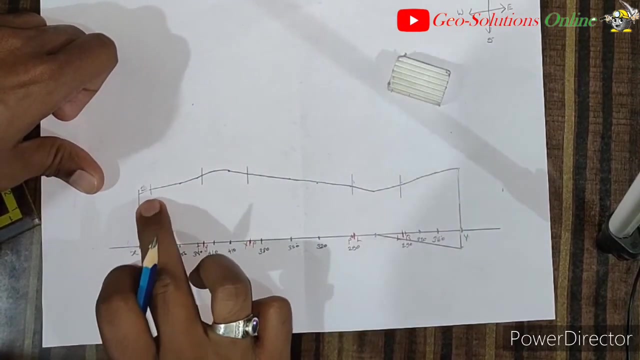 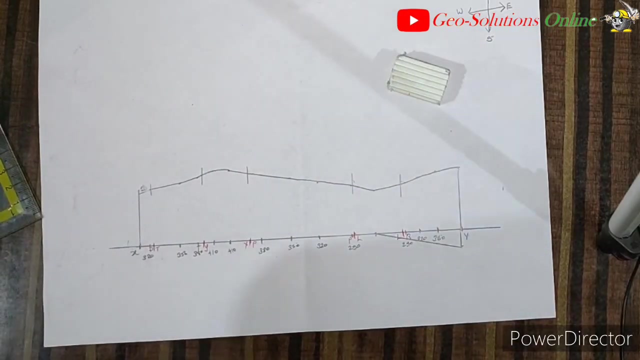 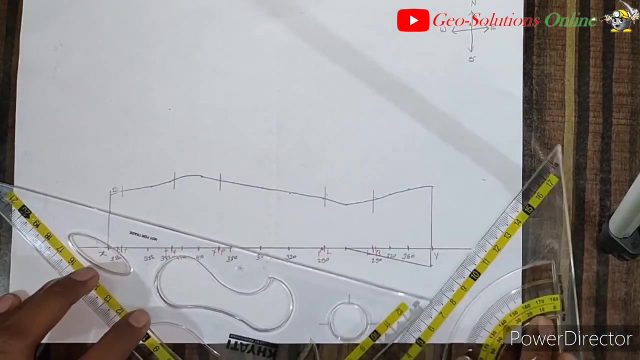 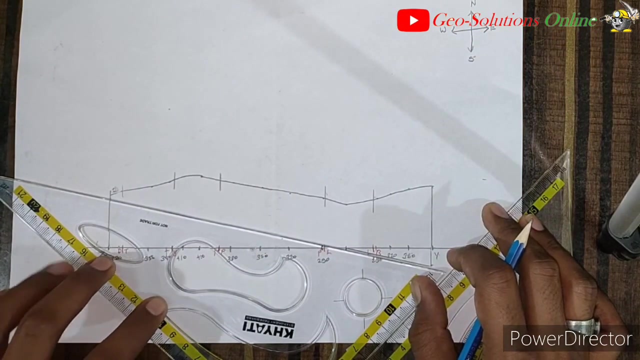 you may use the ruler scale. okay, so here's our bedding. planes are marked- sorry, this is DT- bedding plane T by bedding plane point, YP, PL and LB. okay, how to plot the beds with the help of set square. so first of all, set your set square on this reference line, okay. 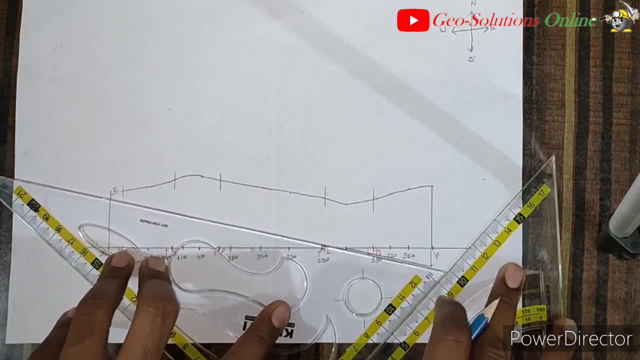 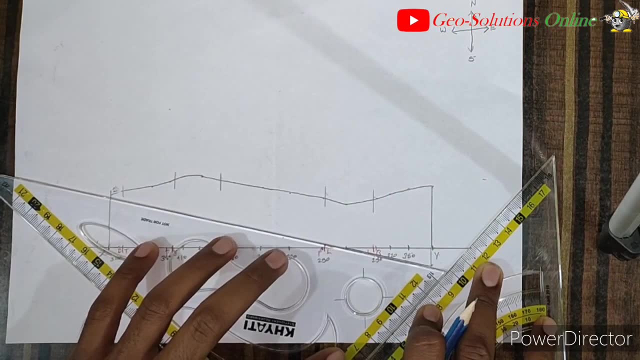 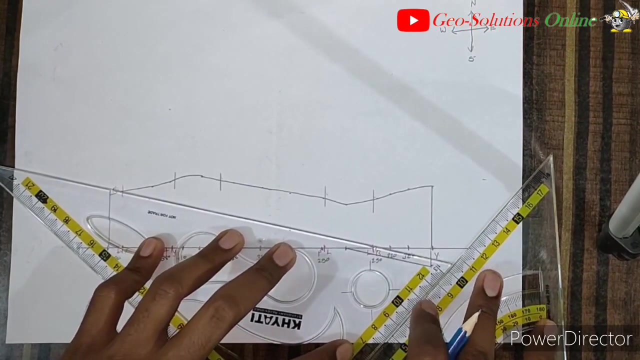 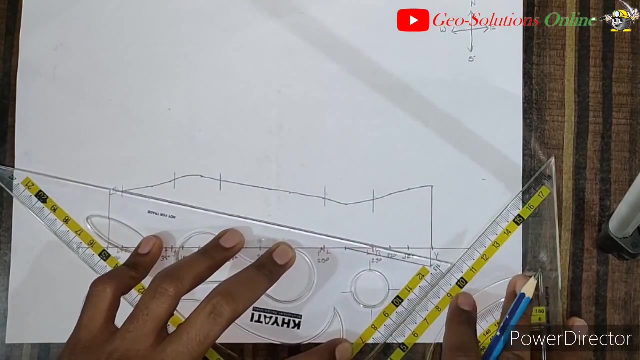 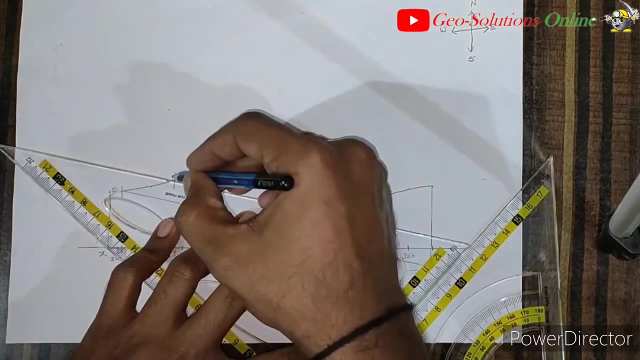 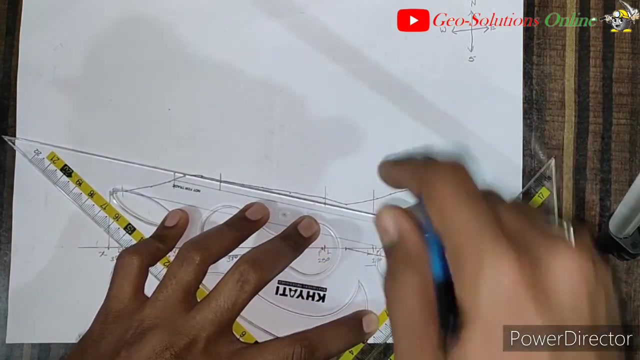 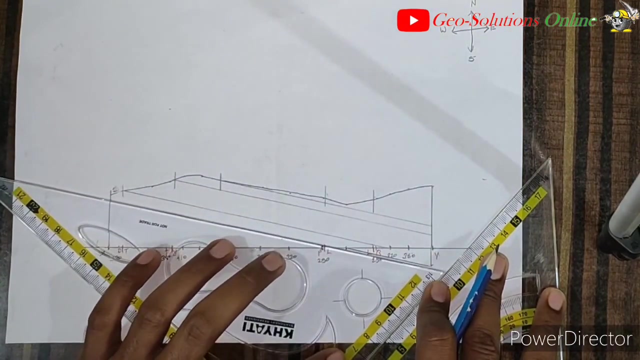 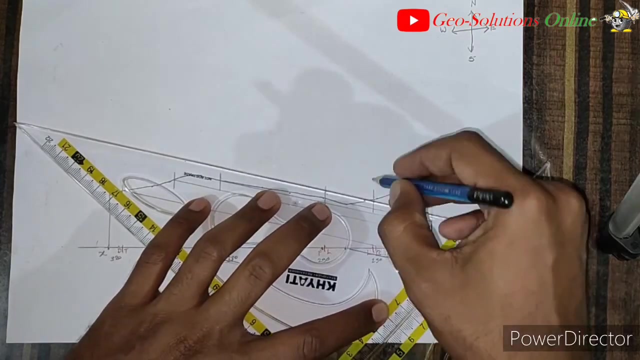 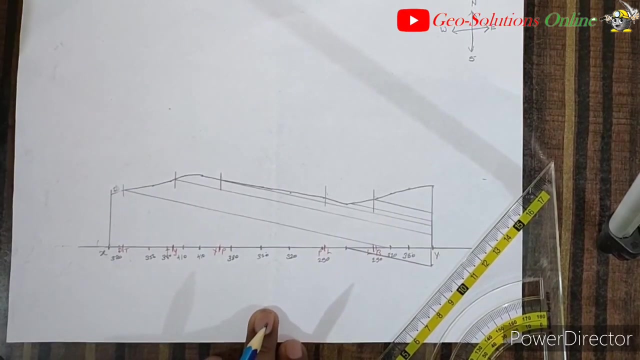 second set square. okay, hold this scale as stable as you can, and this scale slightly move upward as it intersects the point of section of your bed and the bedding point. okay, then slightly move towards next point. so in this way we had plotted all the beds and our section is completed, just. 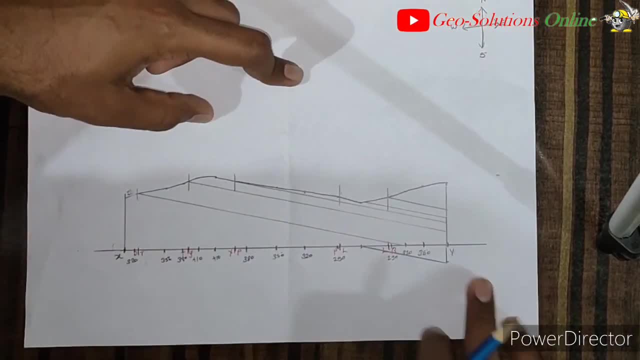 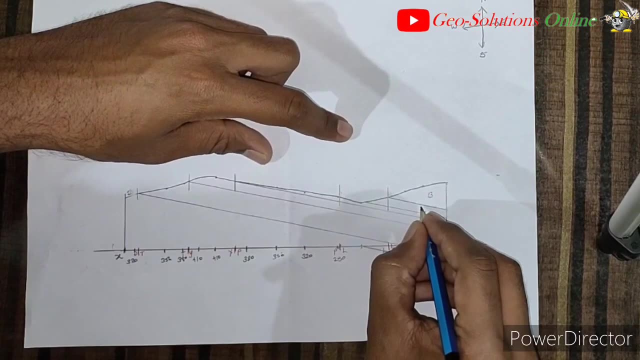 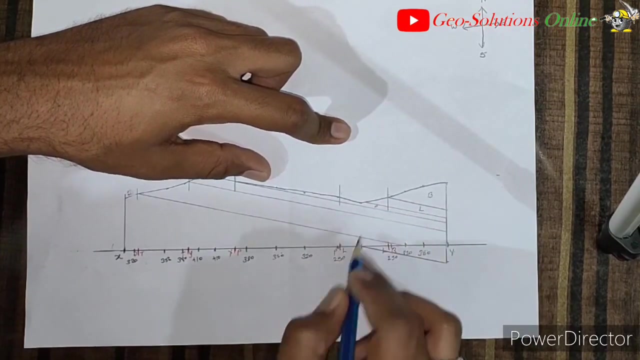 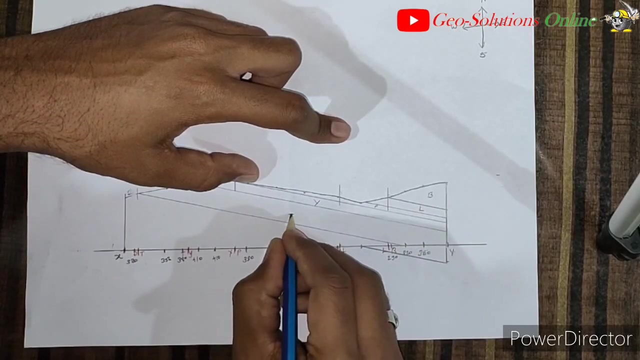 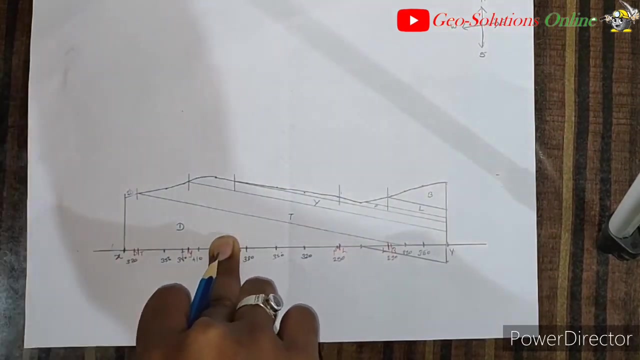 minor things are remaining, we will complete it. so this is our bed B, this is our bed L, this is our bed P and this is our bed y, and this is our bed t and this is our bed D. D is the oldest bed, as we had already studied that in the order of superposition D. 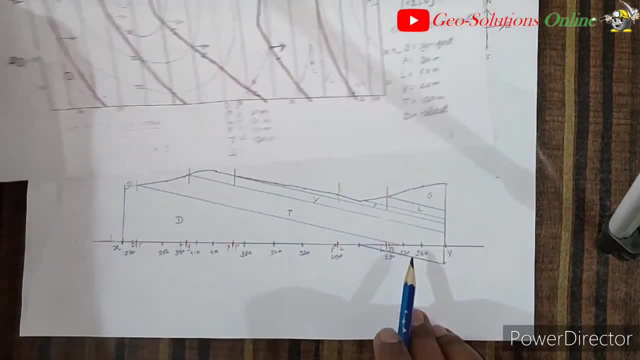 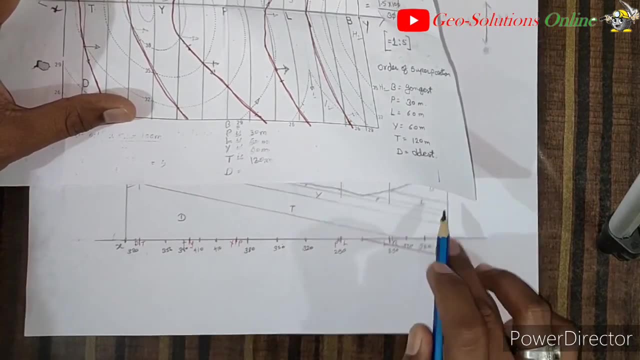 is the oldest bed and the law of the 83, an order of law of superposition, is the bottom of a bed is always one which this is the upper level here. so if you want to join, most bed is the oldest and the uppermost bed is the youngest. okay, so youngest. 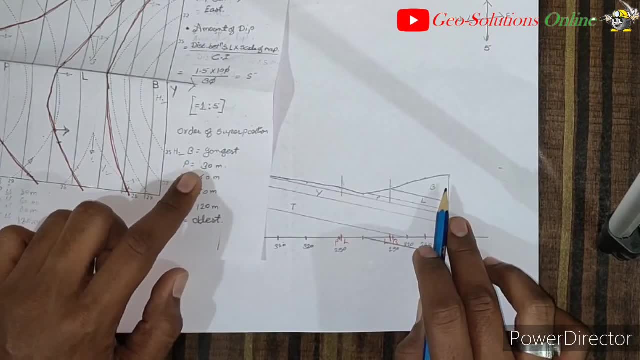 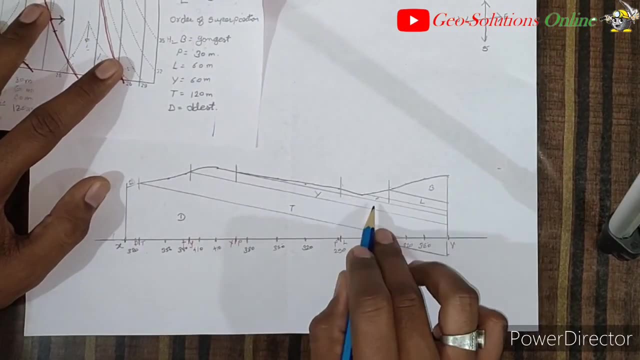 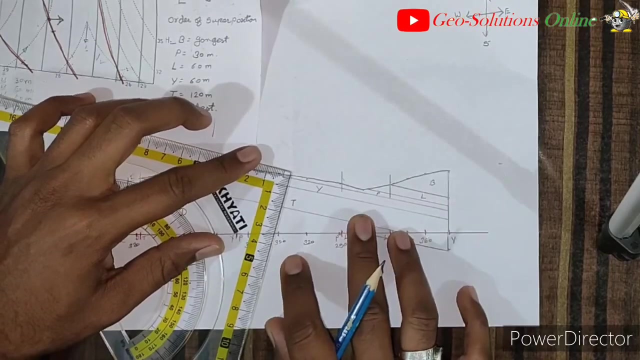 base bed is the B because it is the. it is on top and bottom. most bed is D, it is the oldest bed. this is bed T, bed Y, bed P and bed L and bed B. so if you want to cross check, you can measure the thickness of this bed from here. that is. 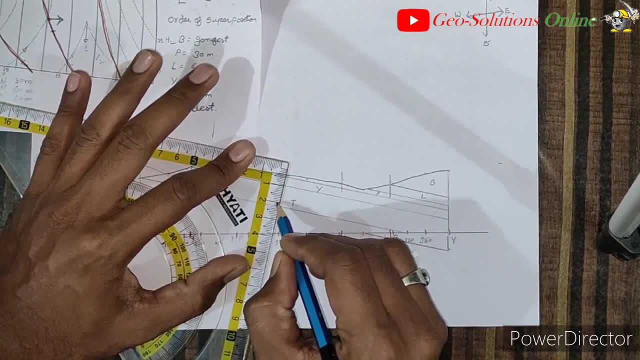 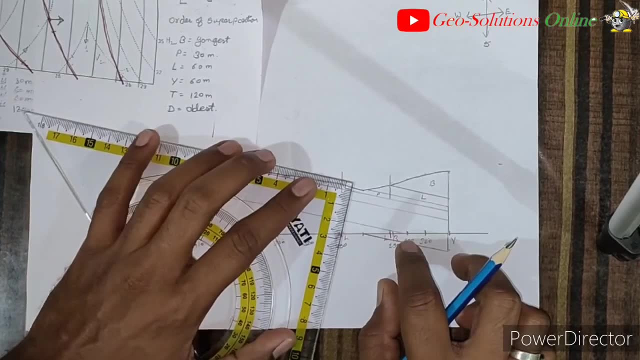 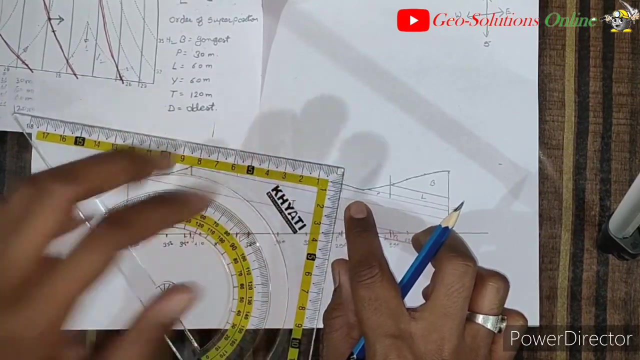 it is clearly showing that it is having 1.2 centimeter thickness. that is, 1.2 centimeter equals to 120 meter. okay, in this way we can also check the thickness of the Y bed. it is showing 6.6 centimeter, that is, 60 meter. 60 meter and. 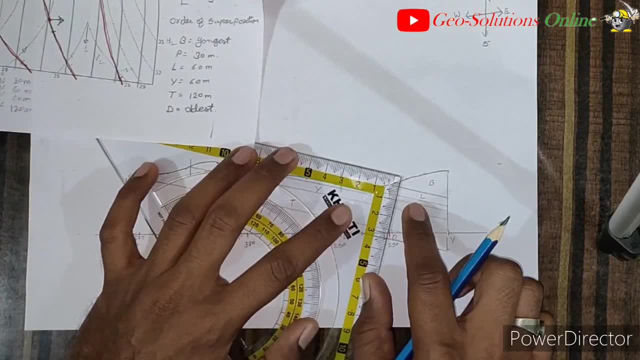 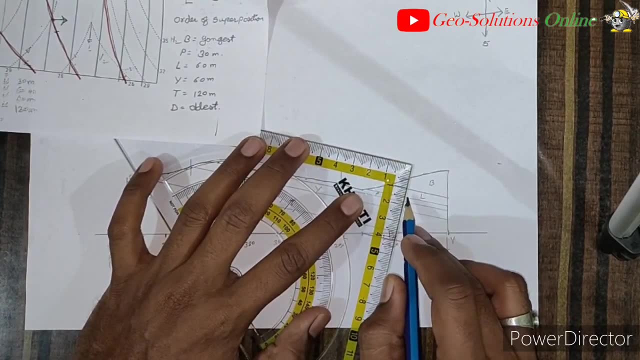 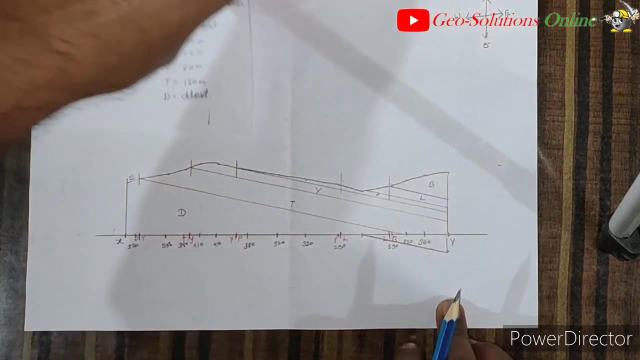 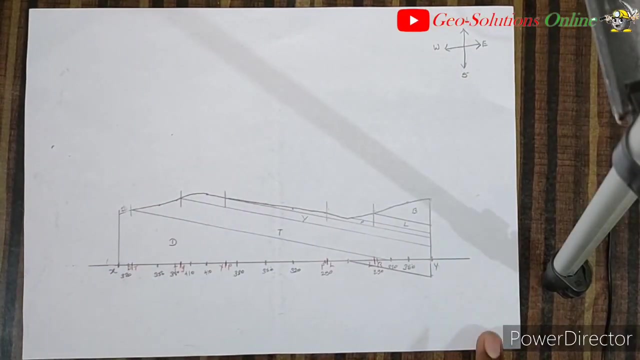 30 meter. okay, so P bed is our 30 meter. you can also check here. so it is showing point three centimeter, it is showing point six centimeter. so in this way we have plotted our cross section of the map number one. so to complete the this section you have to always remember: 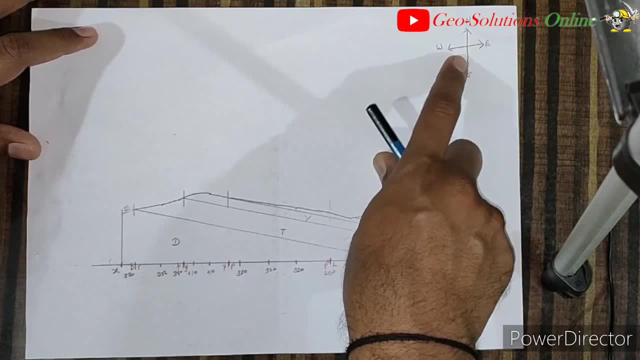 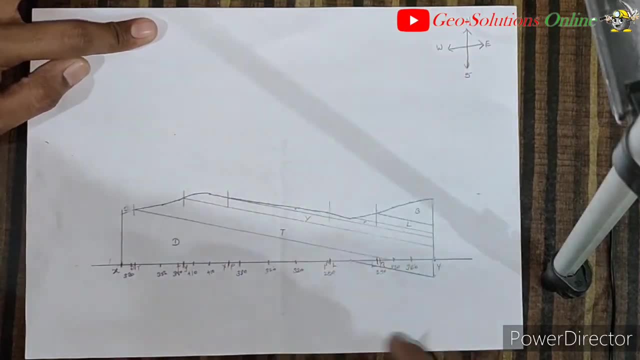 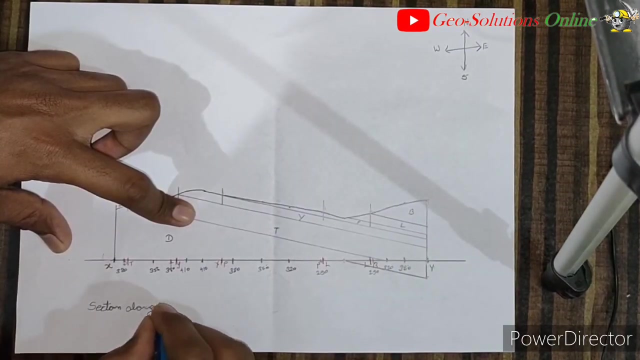 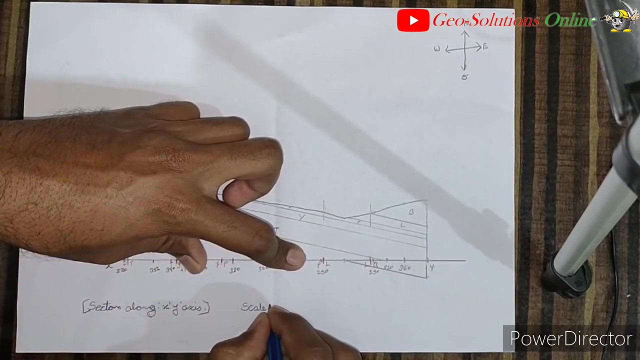 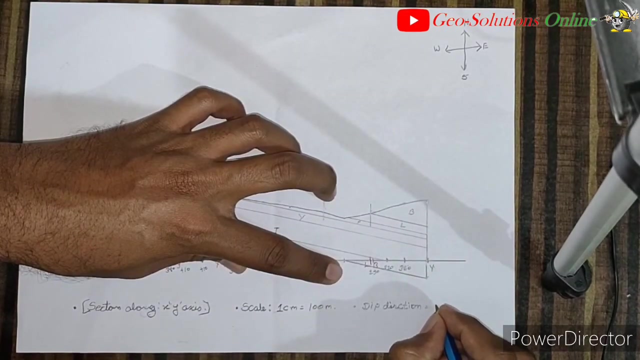 direction is most important. so you have to give the north arrow. okay, if possible, give four direction. okay, then write down always section along X, Y, X, Y axis scale: our scale is one centimeter equals to hundred meter. okay, and deep direction is towards the west, deep direction is towards the east. 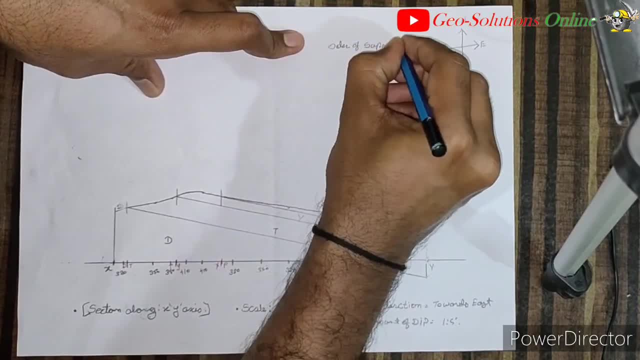 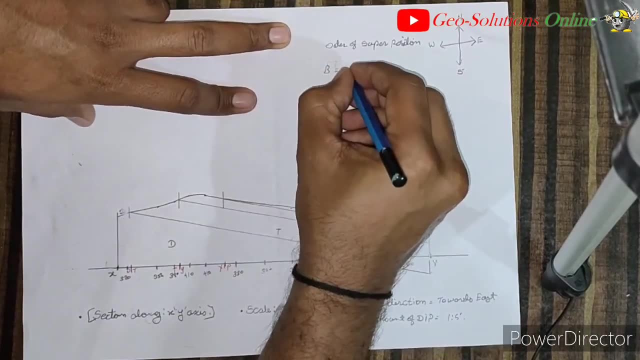 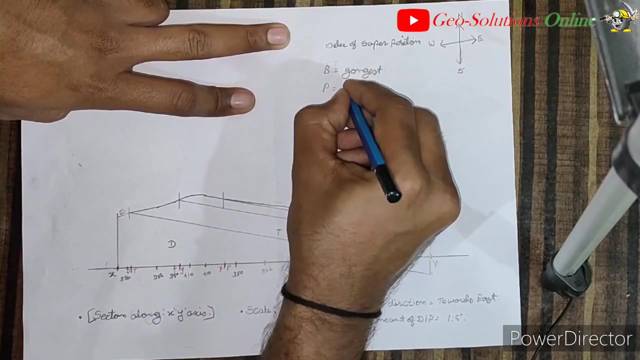 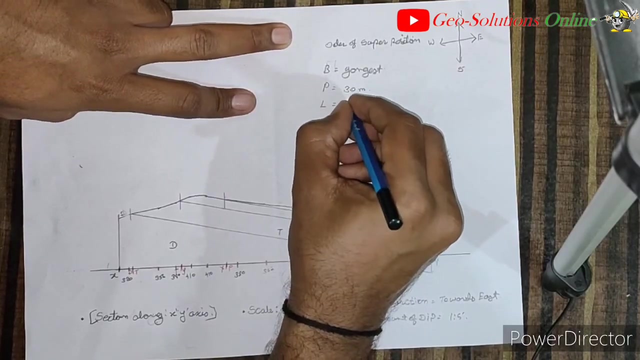 so just do what I am showing you here: north, east, east. table of order of superposition: babies equals to youngest, then bed P having the thickness of 30 meter. so just do what I am showing you here, and deep direction is towards the west. Then bed L having the thickness of 60 meter. 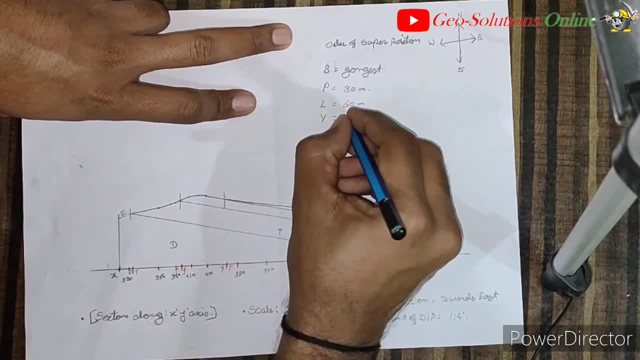 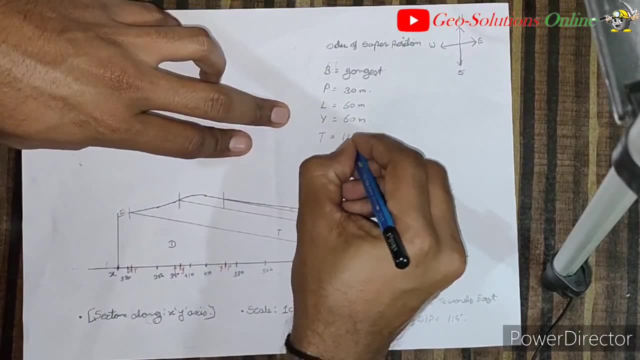 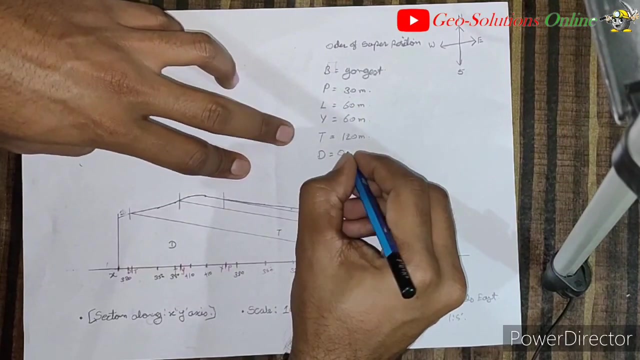 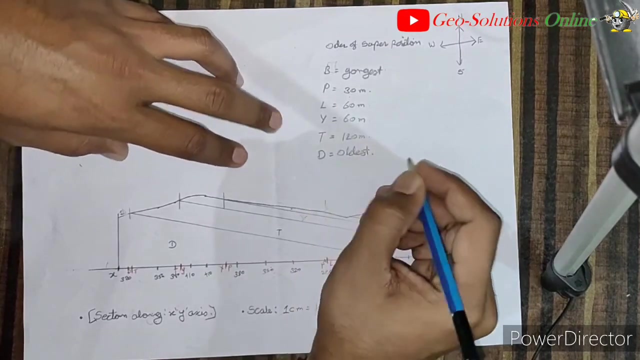 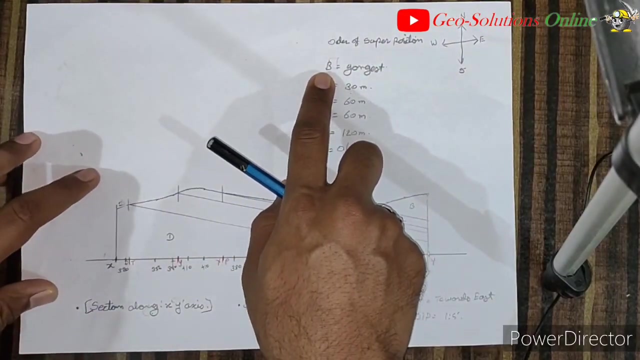 then bed Y having the thickness of again 60 meter, then bed D having the thickness of 120 meter, and bed lastly D having the oldest history, That is, oldest formation. Okay, so this is your order of superposition. you can demarcate this by a different color.